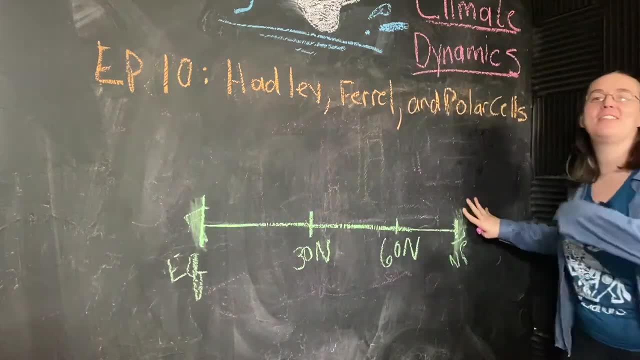 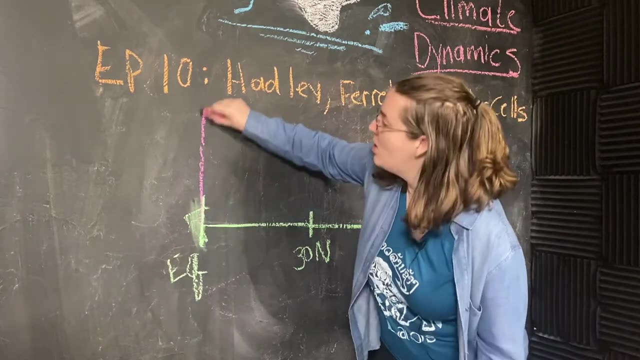 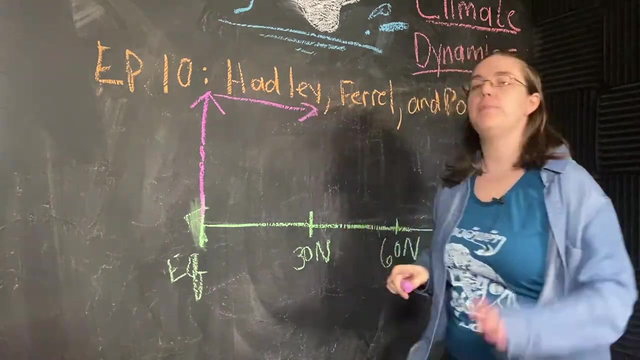 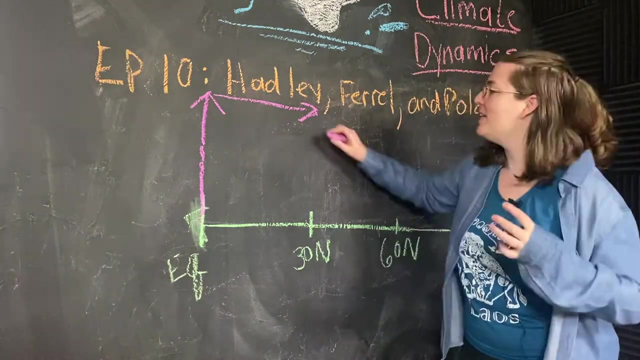 here and it is cold over here and nature does not like that. It wants to mix everything together. So we see air at the equator rise and then it moves northward and because of conservation of angular momentum, this cell breaks down and starts to sink back to the surface around 30 degrees north. and then that would. 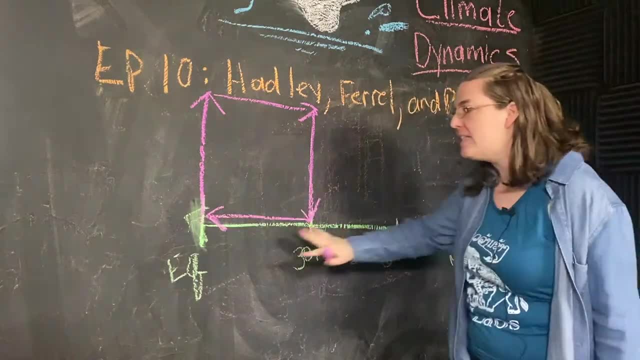 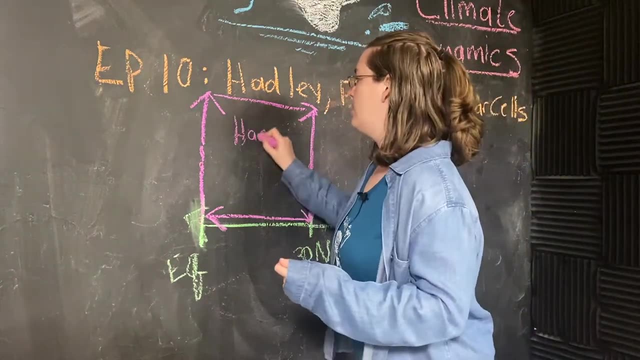 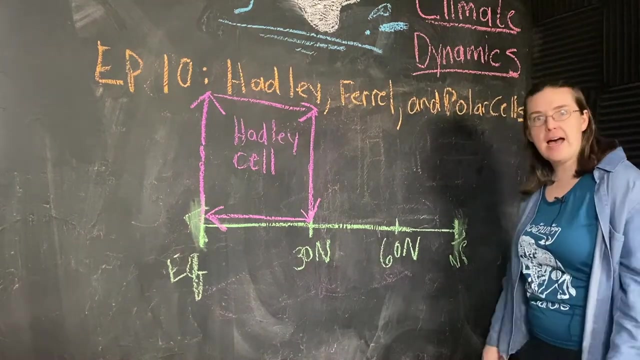 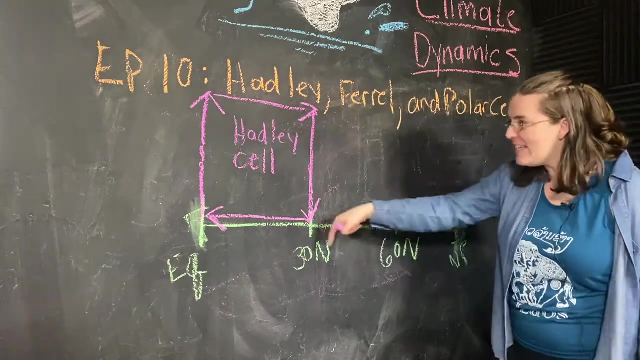 travel. that air would travel back to the equator along the surface, and this is our Hadley cell. Okay, so now let's think about what's going on poleward of this descending leg of the Hadley cell That is. that is a good thing to consider. 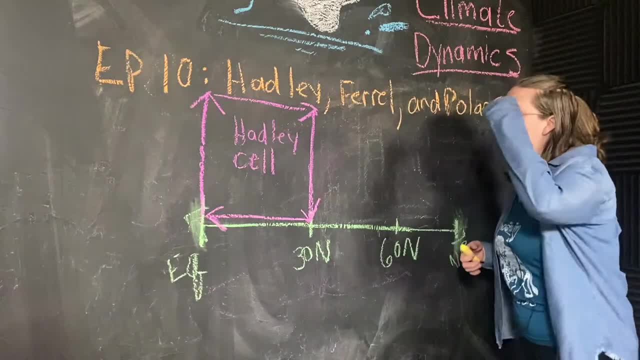 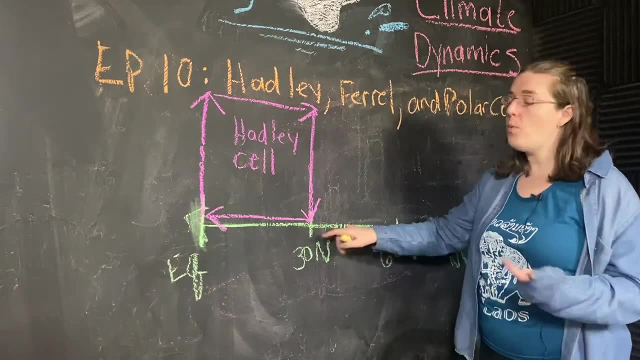 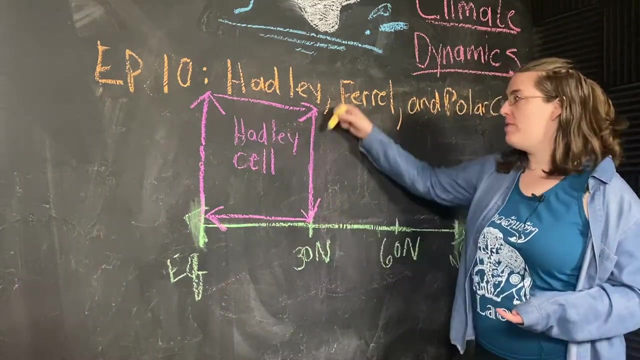 I'm just going to switch colors. Let's use yellow. I like yellow. So we have air that is sunk down to the surface. There's no reason why this air at the should only go this way, right? so some, we've got air coming down. it hits the. 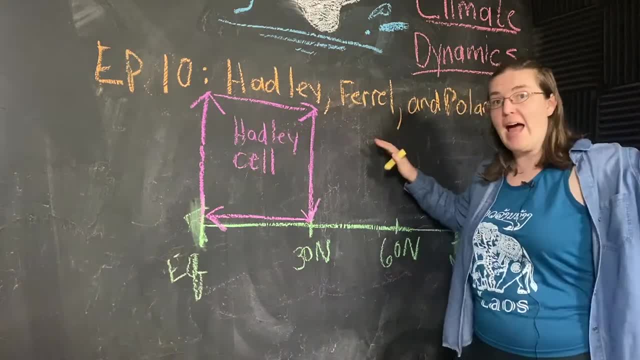 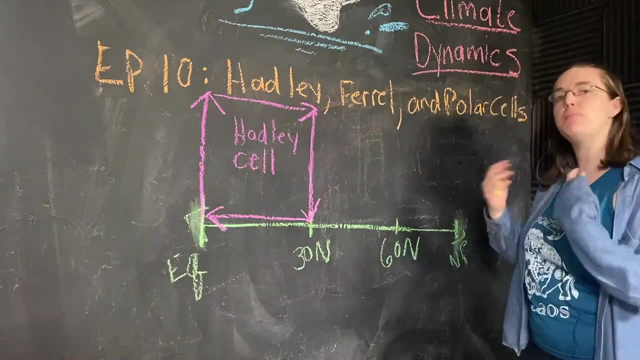 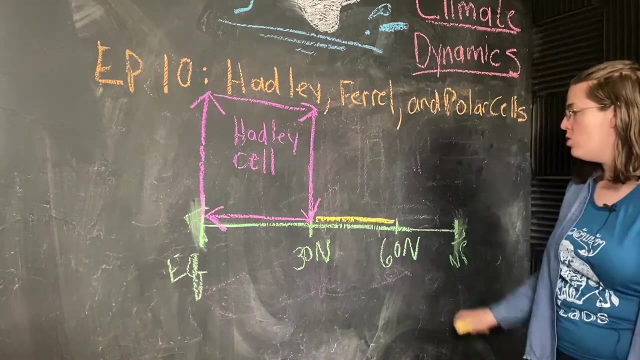 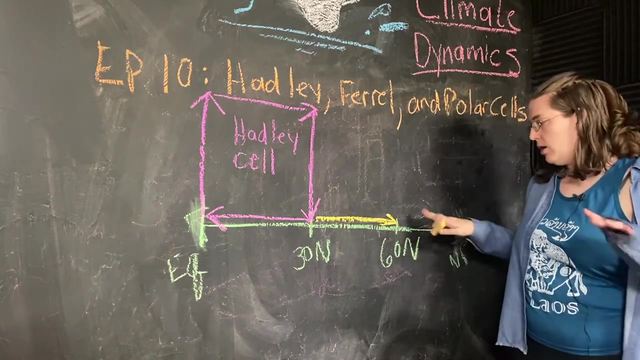 ground it's gotta go somewhere. but it's kind of gonna go splat and go in all directions. but we're just looking along a single longitude or an average picture right now, so we'll just draw that some of this is going to travel north along the surface. that cell it's going to actually start to rise at about 60 north. 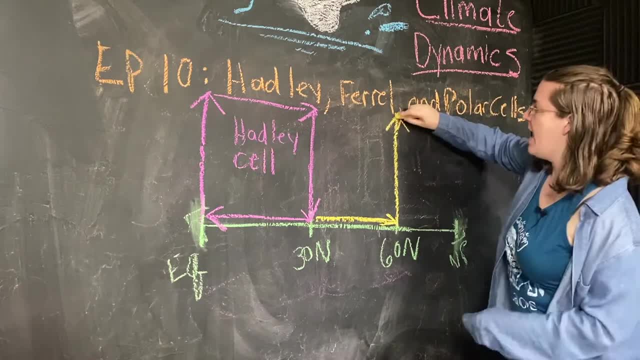 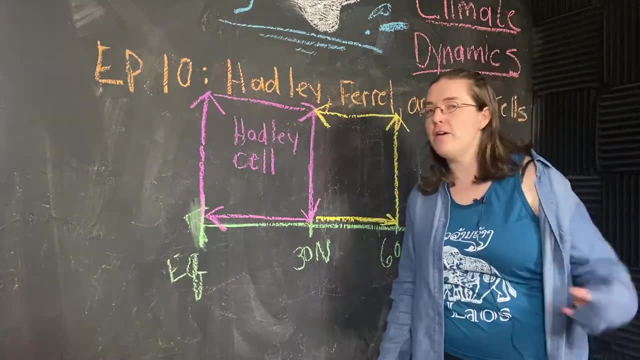 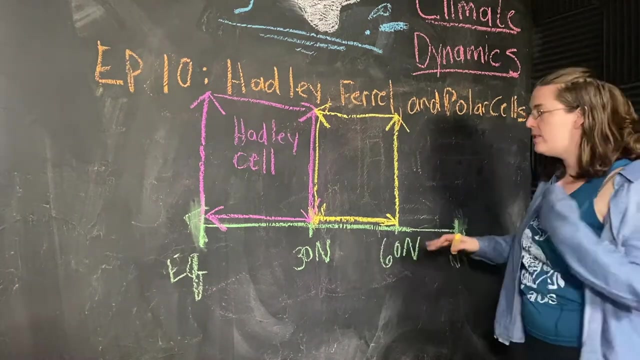 and then head back south. it's gonna kind of run into that poleward arm of the Hadley cell and sink. so we have this type of circulation from 30 to 60 north. this one is going to go north along the surface and then head back south. it's. 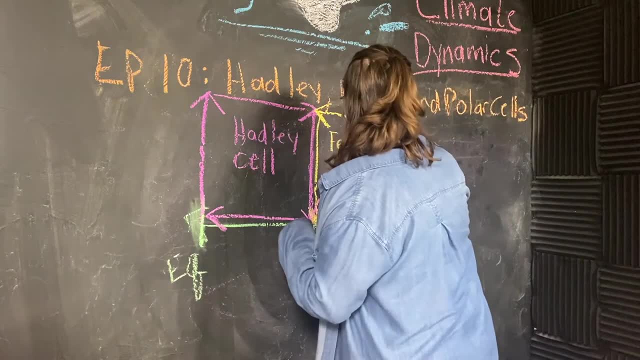 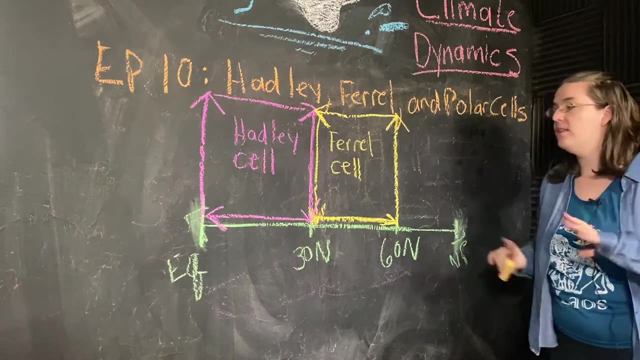 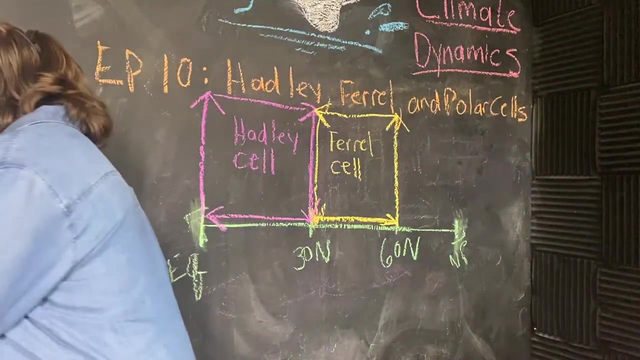 gonna go south along the surface and then head back south. it's gonna go south. this is called the ferrule cell and, last but not least, is going to be the polar cell. so I'm going to change colors again. maybe let's use a nice blue, because it's 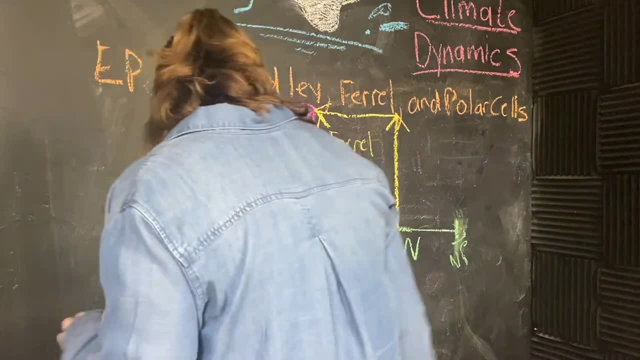 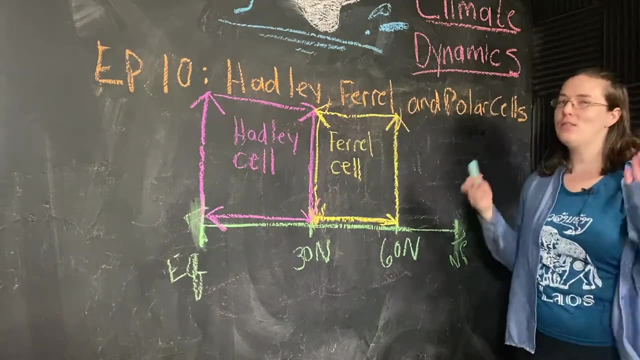 cold up over the pole. there's my blue chalk. okay, same thing. as this air is going up, it's not only going to go to the south. it's not only going to go to south, it's not only going to go to the north, it's not only going to go to the. 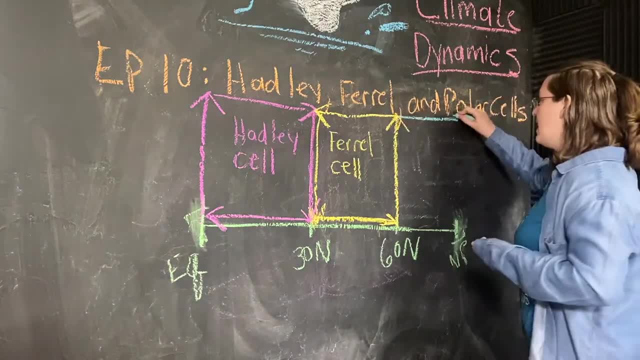 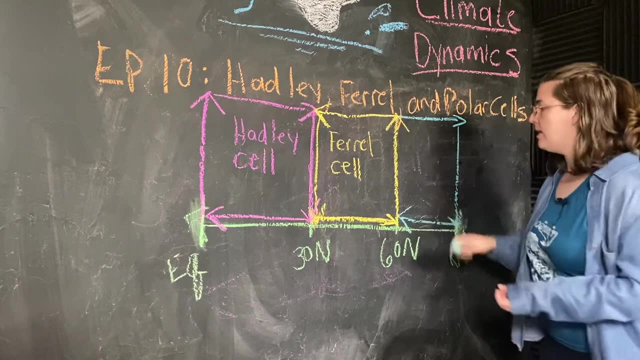 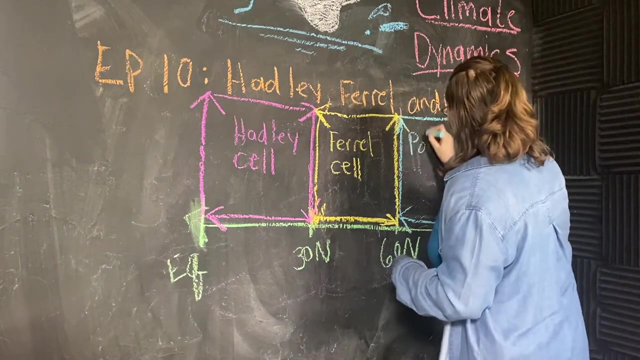 north. it's not only going to go to the south, it's not only going to go to the equator word. there's no reason why some of it can't come back up north. we would sink and then return back here rising air. that way, here is our polar cell, and 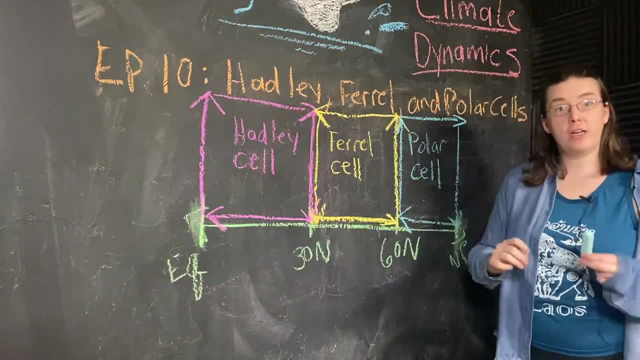 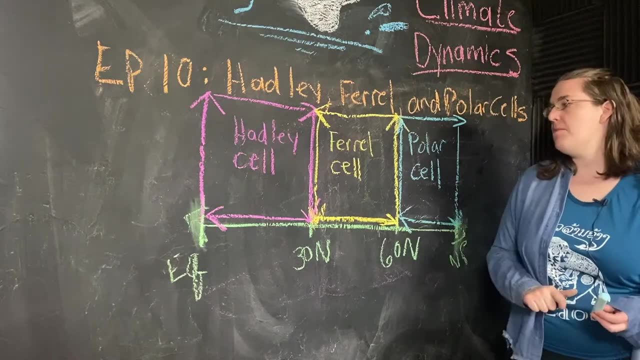 so we get. we know that the Hadley circulation right was driven by this desire to move my warm error from here, from the south up north, and then head the equator poleward. but its size was set by angular momentum. Same is going to be true of 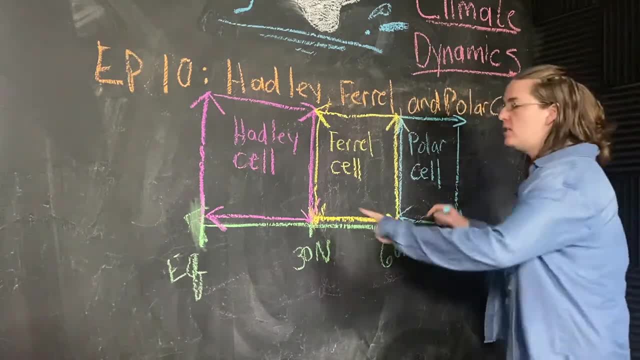 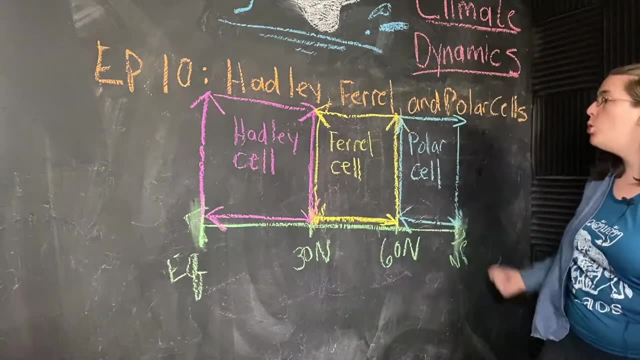 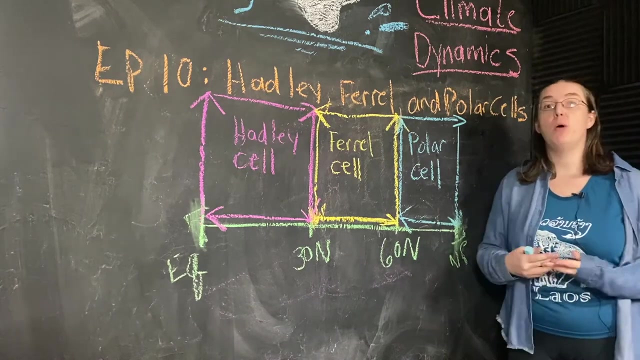 the ferrule and the polar cell Collectively. what these three circulating cells do is they work to transport heat from the equator to the pole, And we get the three different ones because we are balancing conservation of angular momentum with that driving force of it being hot here. 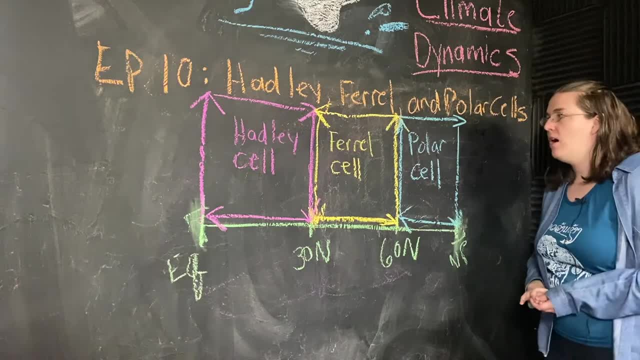 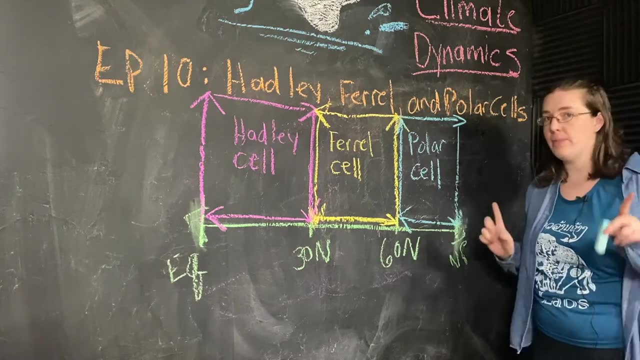 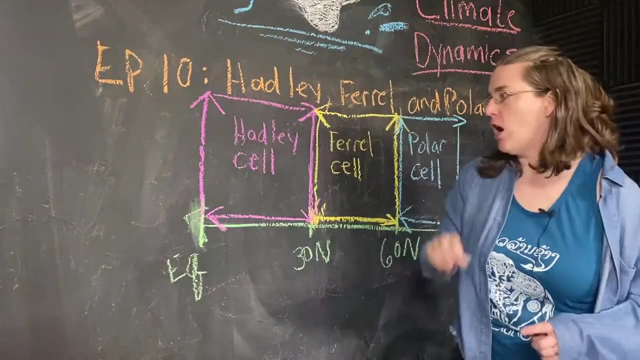 and cold here. So this is our basic structure. Now let's talk about what this means for global weather patterns. So we talked about this a little bit in the last video. I'm going to use some white chalk to denote like relative surface pressure. 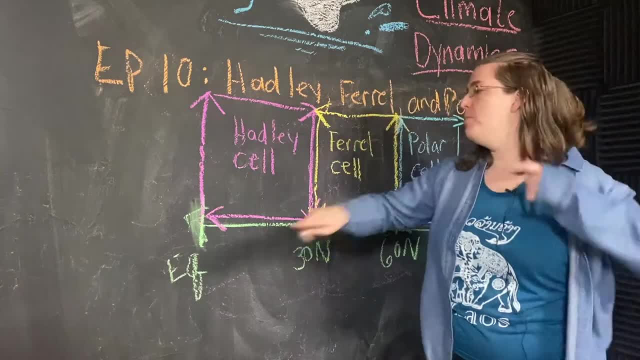 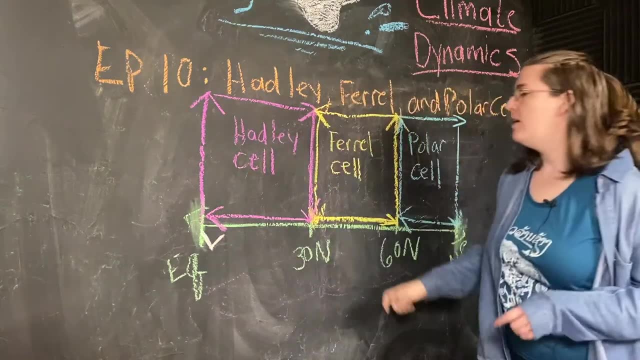 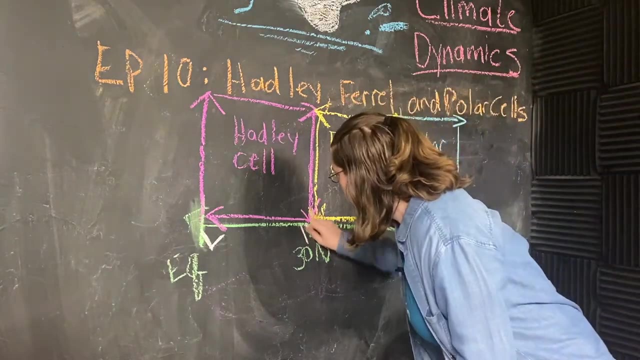 So anywhere we have air moving away, moving up right, we're going to see low surface pressure. and anywhere we have air coming down, pushing down on the surface, we're going to have high surface pressure. So we'll have low pressure at the equator, high pressure around 30 north. 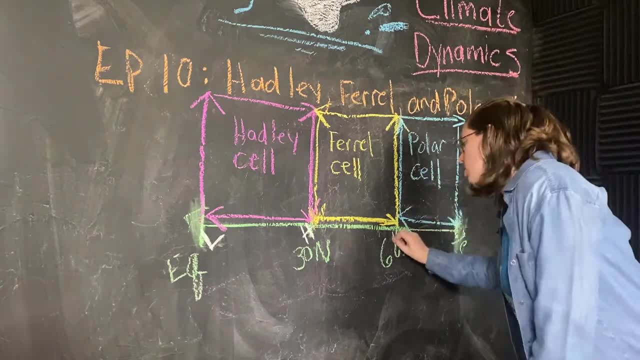 We've got air running away from the surface at 60, so that's going to also be a low pressure 60.. If we've got air running away from the surface at 70, that's going to be another 30.. Yeah, So there's differentribами, This loop load of circuitry. we close it down towards the ну. 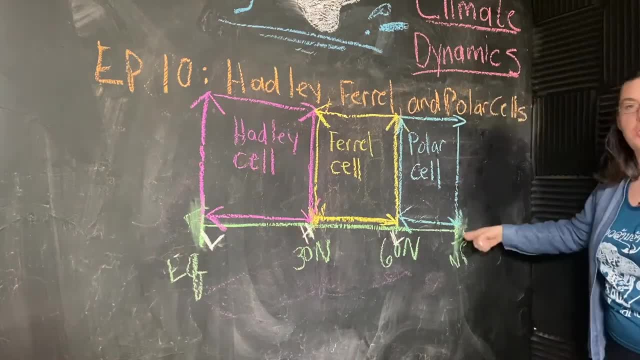 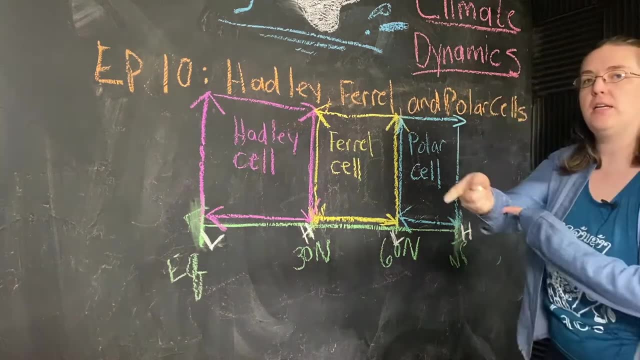 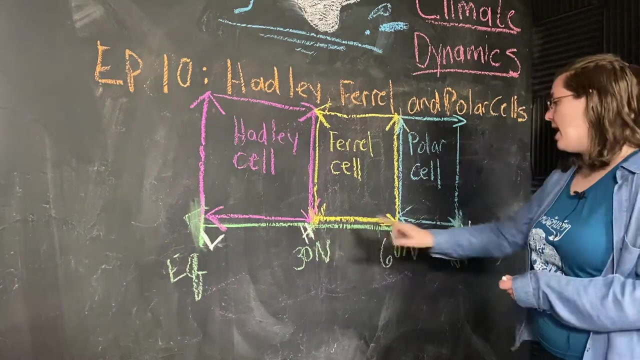 system And we'll have high pressure here at the North Pole. And this is, if I forget to say this- this is all reflected into the southern hemisphere. It'll just be a mirror image. So we have net lows, high, low, high. And then what does that mean for clouds? Well, 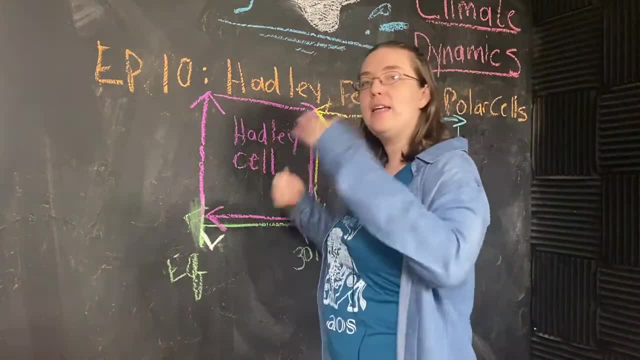 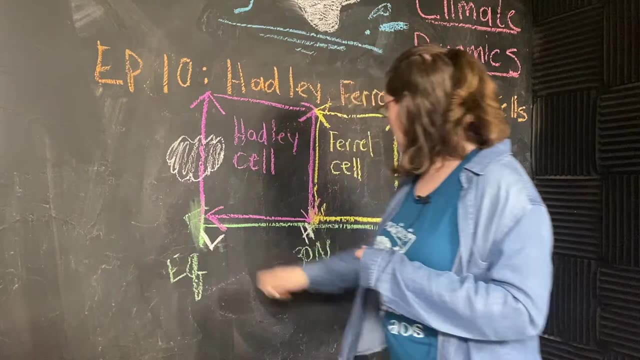 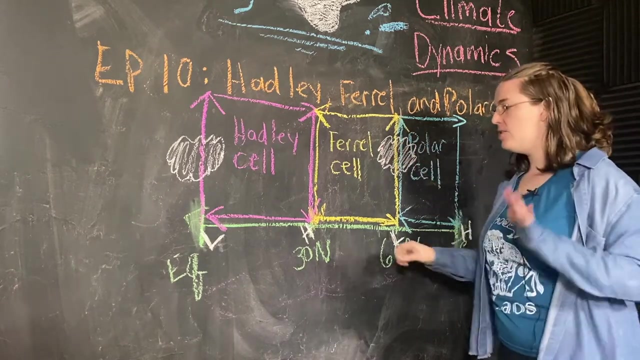 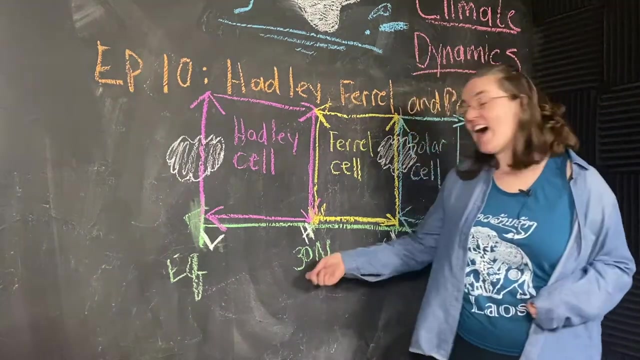 I want you to start thinking that low pressure net rising air is going to be related to clouds. So let's draw some fluffy clouds here at the equator, here at around 60 North, And no clouds here around 30 North and here at the North Pole. And we saw last time that if you track 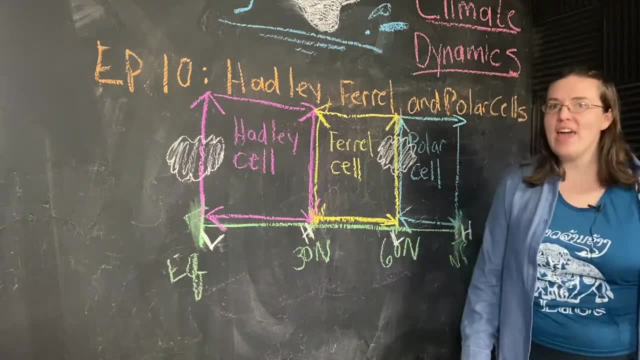 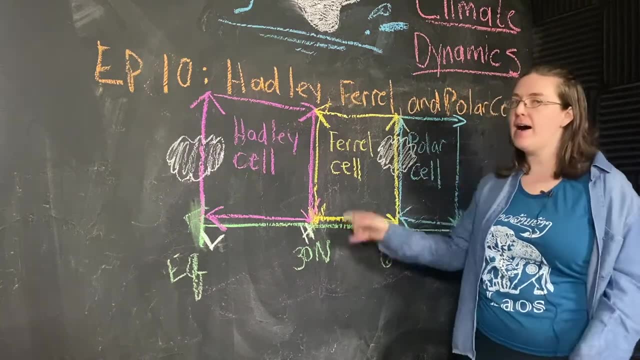 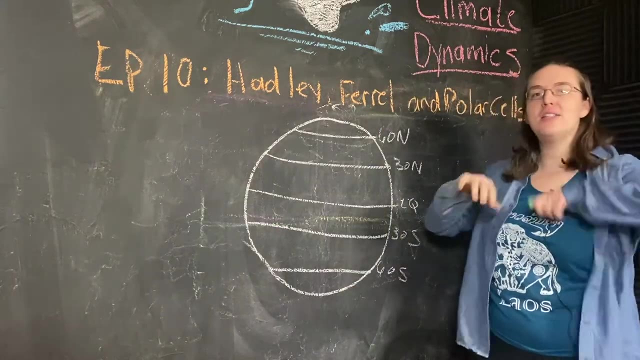 about 30 degrees around the globe, you run into a lot of desert regions, which is exactly what we would expect from this global circulation picture of high pressure. Oh, I'm sorry. Okay, Okay, team. So let's talk about what surface winds we get because of those three. 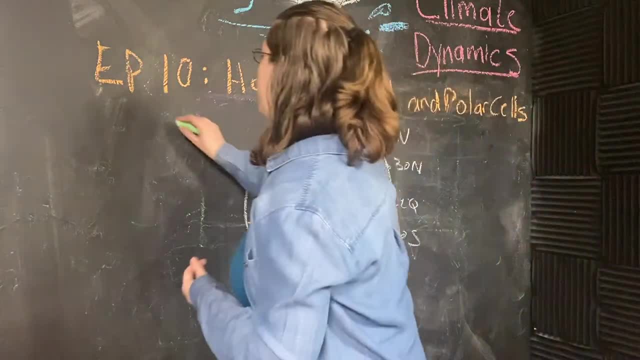 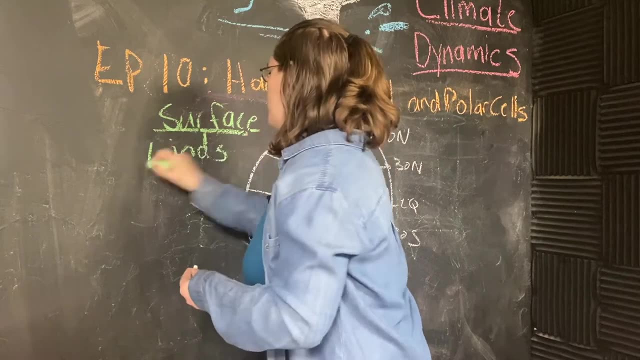 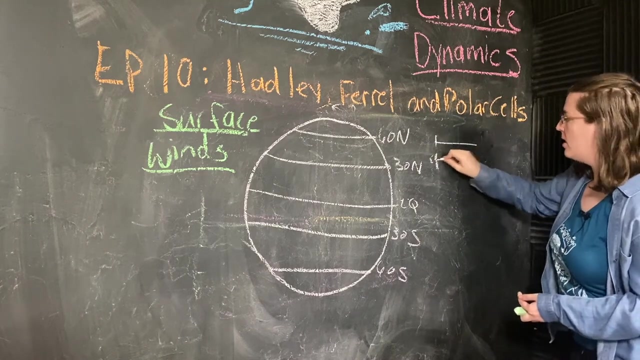 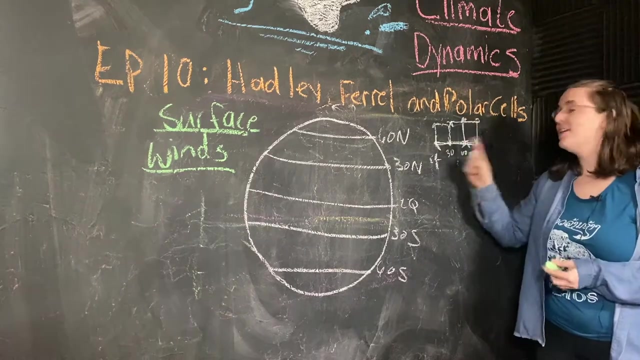 solids, our Hadley, Polar and Farrell cells, Surface winds. As a little reminder, let's just draw a sketch over here: If here's our equator, here's the North Pole. This is 30,, 60.. Because of the Hadley, Polar and Farrell cells. 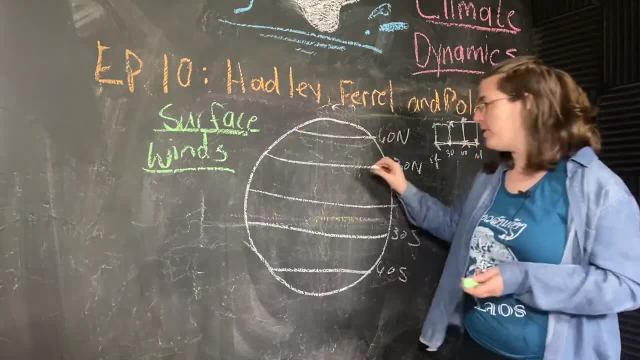 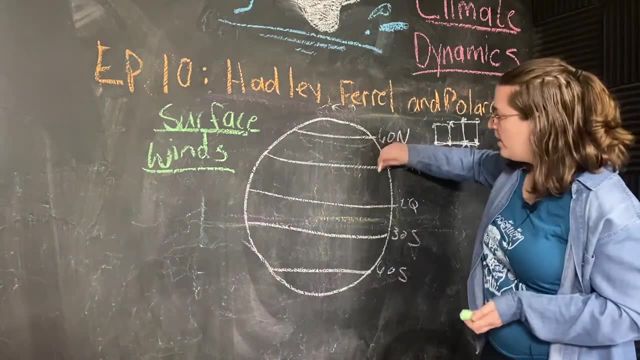 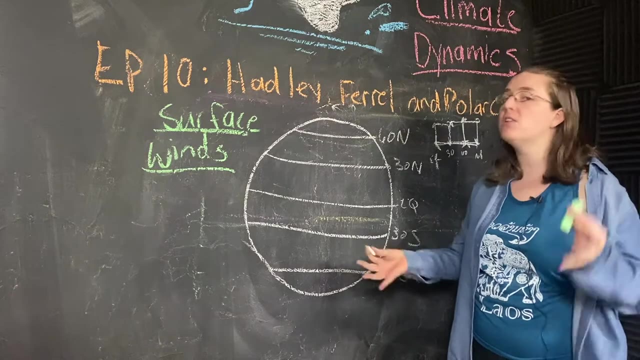 Surface winds are going to be going from 30 towards the equator right. The air travels along the surface back towards it. But we get a really interesting thing from the Coriolis effect, which is rooted in conservation of angular momentum, And what that is is. this is going. 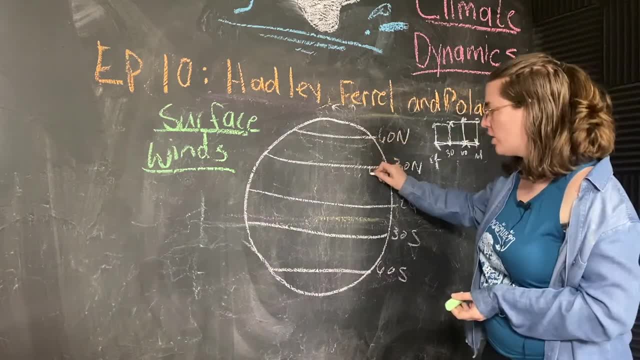 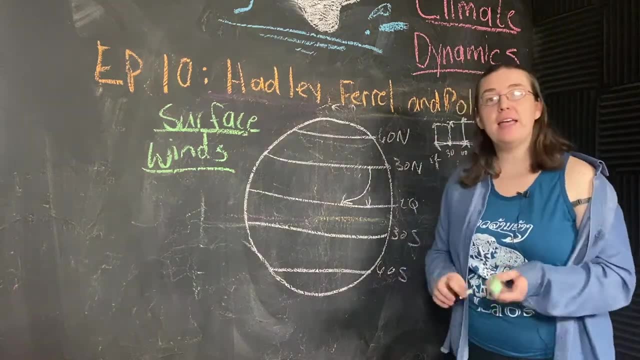 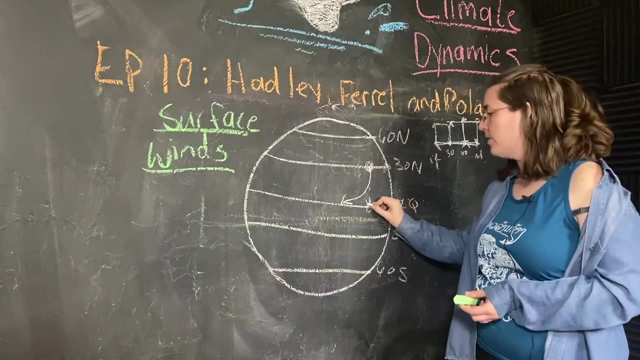 to get deflected. If the air parcel is trying to go like this, it actually gets deflected to the right, Okay, Okay. And one way to think of that is: an air parcel here has to be moving slower than an air parcel here. 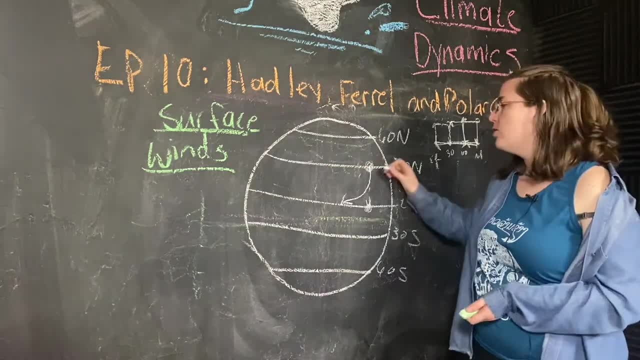 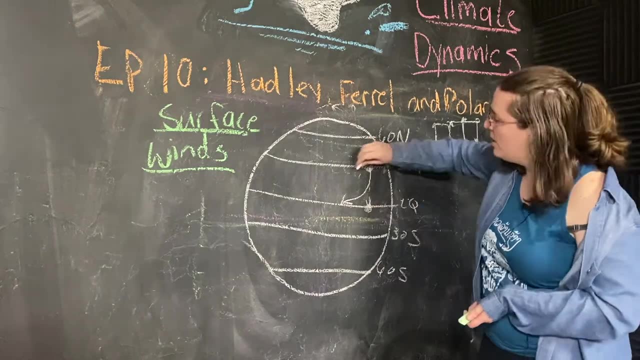 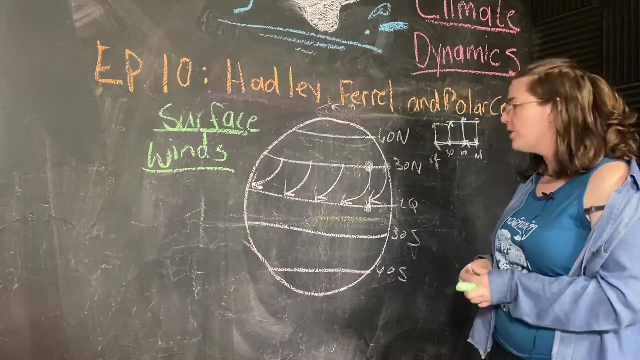 in order for them to be moving with the Earth at the same rate. So if I try to just bring this guy down, he's going to get deflected behind the parcel that was already here. So this goes like this: There's my surface winds, And 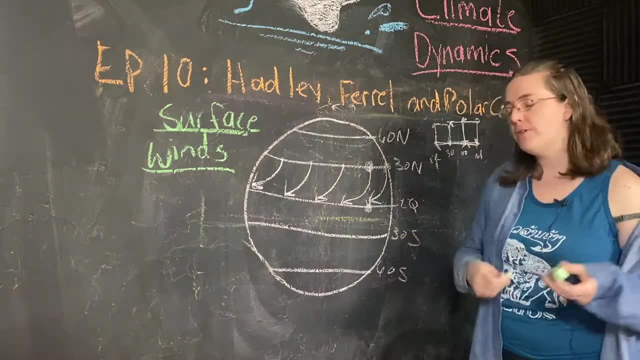 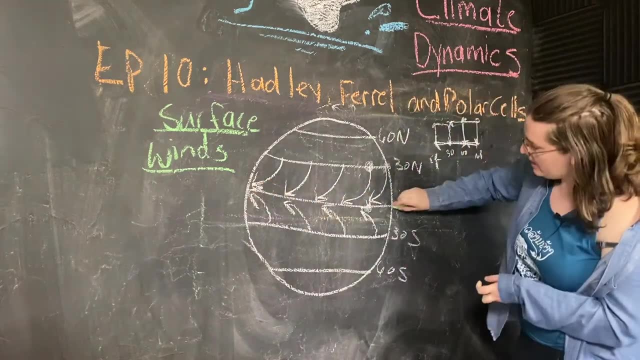 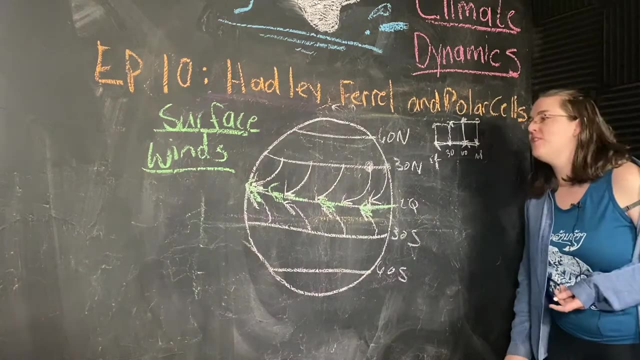 in the Southern Hemisphere it's deflected to the left for the same reasons. So it goes like this. So we get these really strong winds at the surface there in the tropics. These you might know have heard called the trade winds. These were very important. in the days of sailing ships, So you wanted to be able to travel along the equator. You're going to go a lot faster, Okay. So, unlike if we're near 30 degrees north, where we would have air trying to move to 60 degrees north on that surface leg of the ferrule cell, 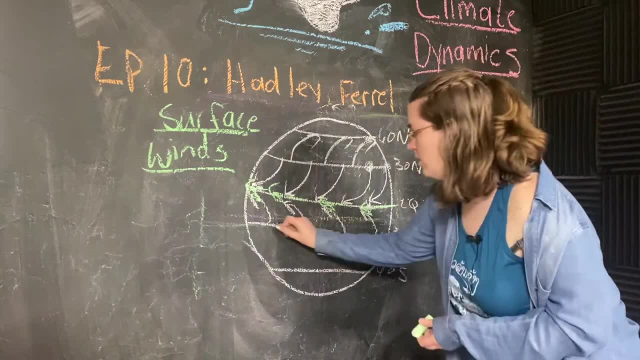 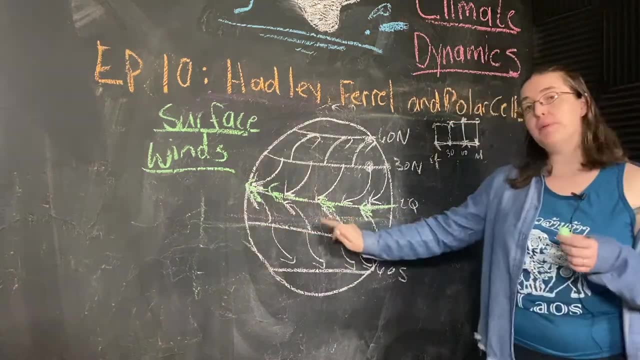 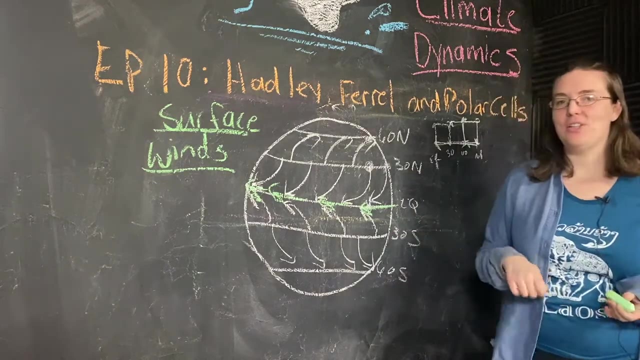 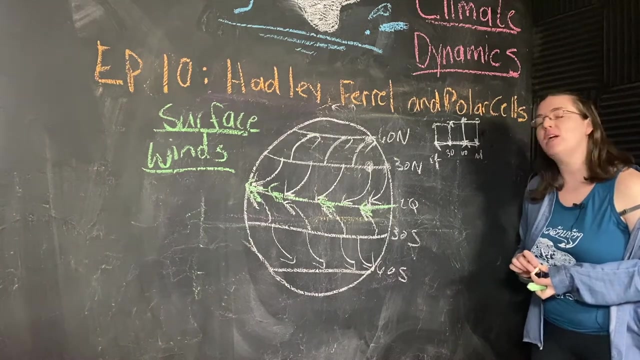 We get There we go, So we get winds going in like opposite directions at the surface: around 30 north, 30 north and the south. Those were called the horse latitudes, or possibly the doldrums is a term I have heard. These are not very great places to sail. What I do also want to say is that these 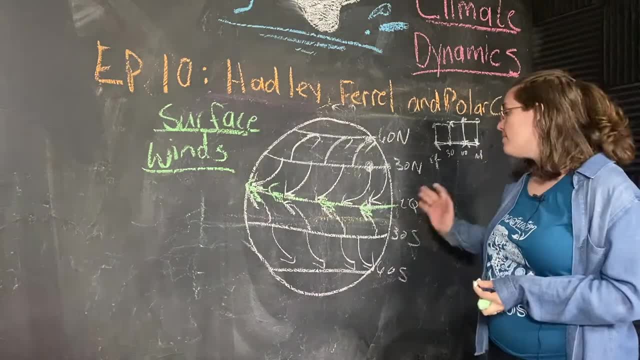 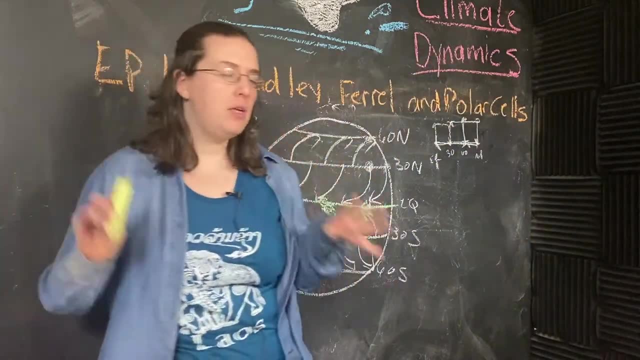 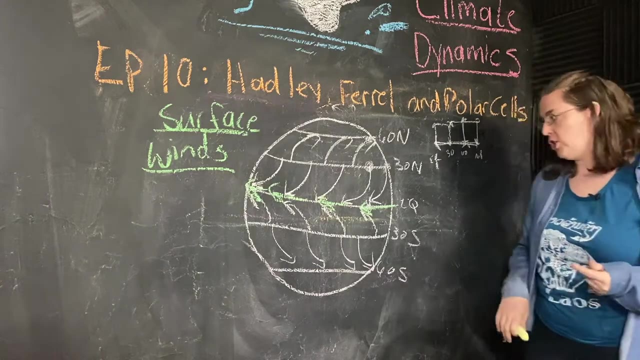 three cells- the Hadley, the feral and the polar cells- break the earth up into these three main regions that we meteorologist-type humans like to talk about. So basically, the weather behaves very differently in those three regions. So here, between plus and minus 30 degrees. 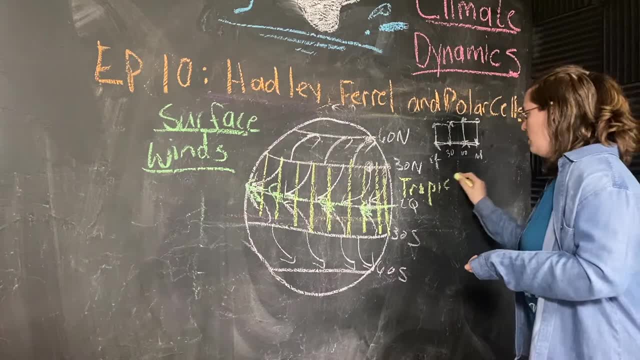 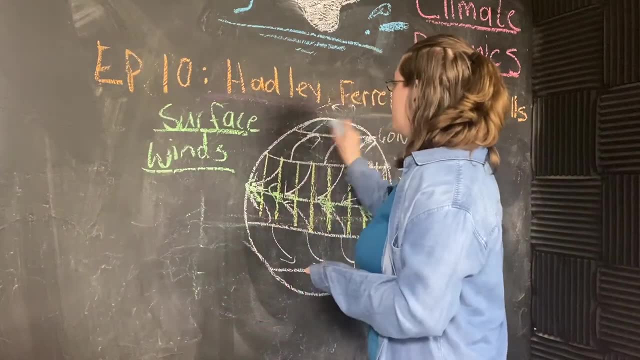 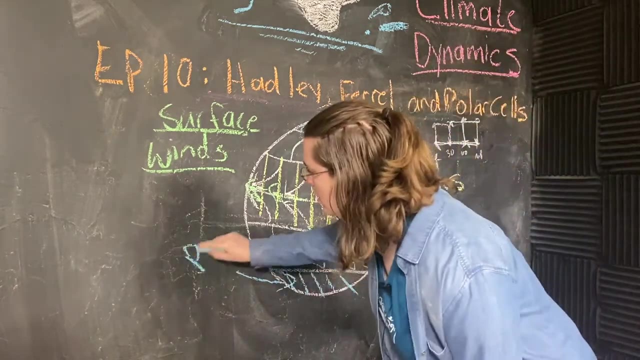 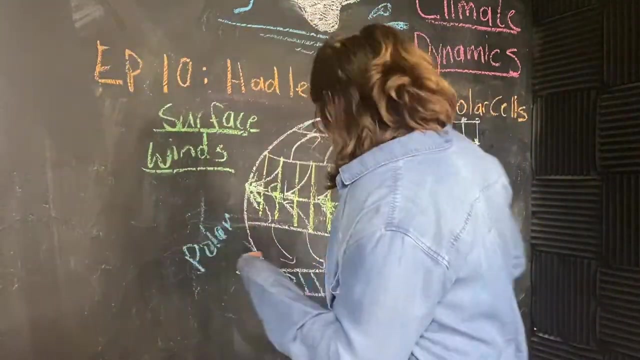 these are the tropics. There's the weather in the tropics. We'll do blue if we look north of 60 degrees or south Of 60 south. those are the polar regions Very cleverly named, And, last but certainly not least, where arguably the most interesting. 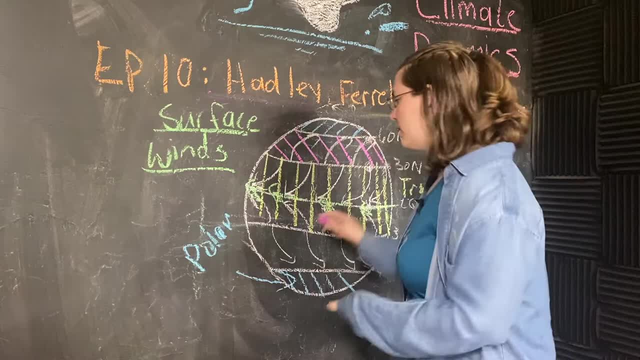 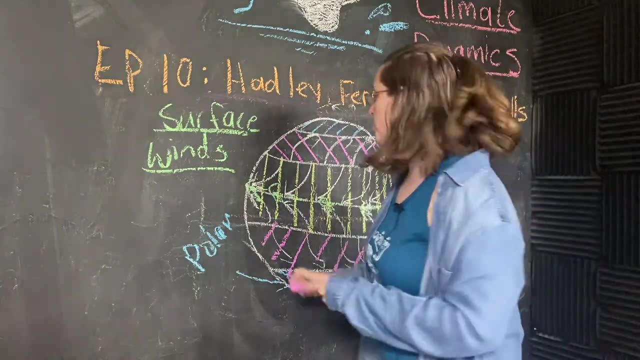 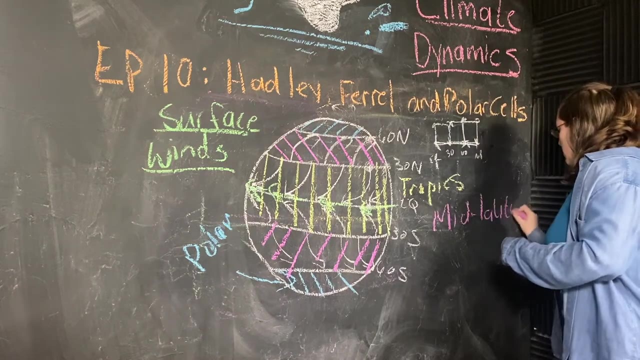 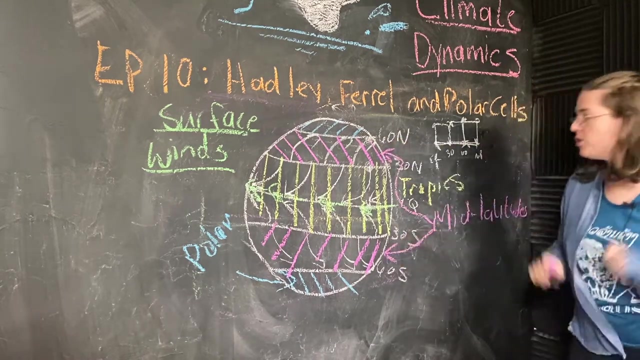 weather occurs is between 30 and 60 degrees in either hemisphere, And those are referred to as the mid latitudes. So where can I write that? Here we go, Mid latitudes. So the mid latitudes weather gets very interesting. right, There's a reason we can get.